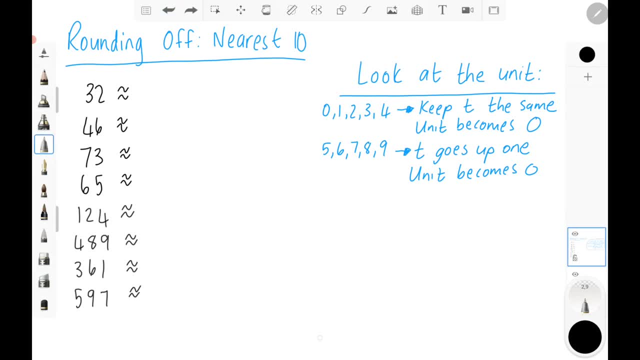 So it's the 10's place in every number. So we've got to look at whatever number is in the 10th. So I'm just underlining all the numbers, that are, all the digits that are in the 10's place. 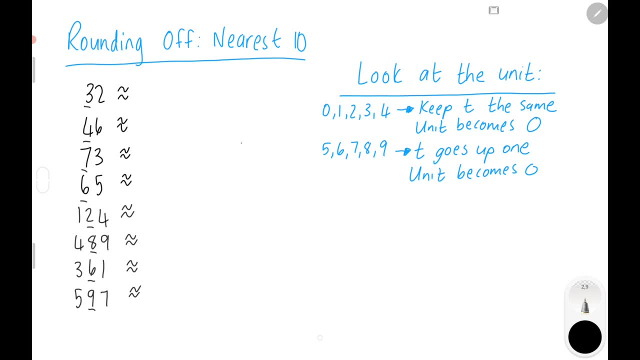 The 10 needs to change. Sometimes it changes and sometimes it stays the same, depending on the circumstances, But we always need to look to the right of whatever the nearest is that we are trying to round off. In this case, if it's nearest 10, we've got to look to the right of our 10.. 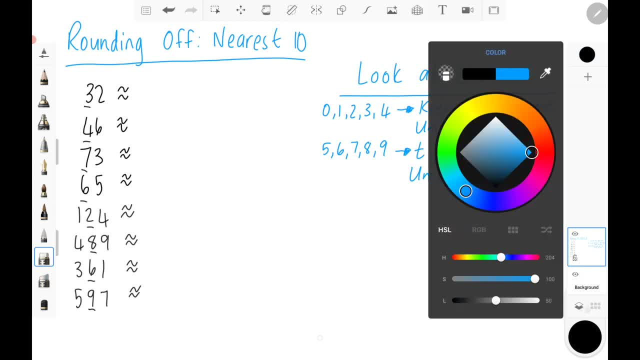 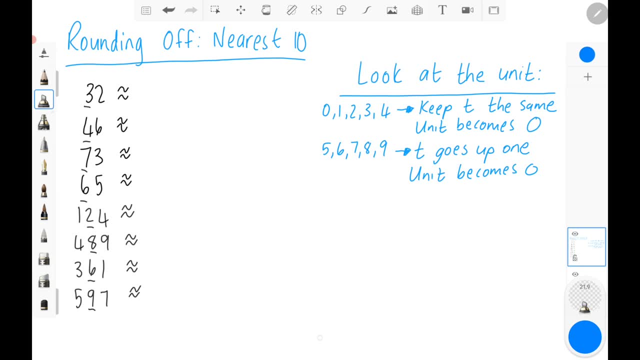 And that number to the right is what I always say. It's the buddy that helps us to round off, okay. And what place is sitting to the right of the 10's place? Well, it's the units, okay. So every time we're doing rounding off, if it's nearest 10, we look to the right, which is the unit. 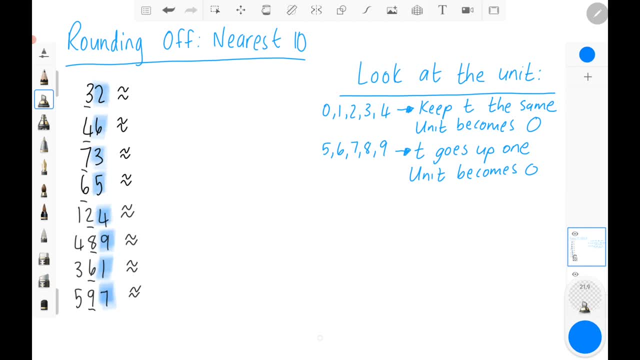 If we're doing nearest 100, we look to the right, which is the 10's place. If we're doing nearest 1000, we look to the right, which is the 100's place. So, no matter what it is you're changing, look to the right. 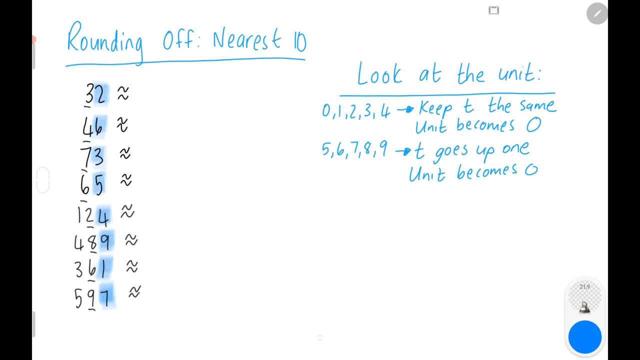 And that place will help you determine what to do with the nearest. So I've highlighted your unit to show you that you're going to use the unit to decide what to do with the 10.. And the whole point of this rounding off to the nearest 10 thing, if we think of something on a number line. 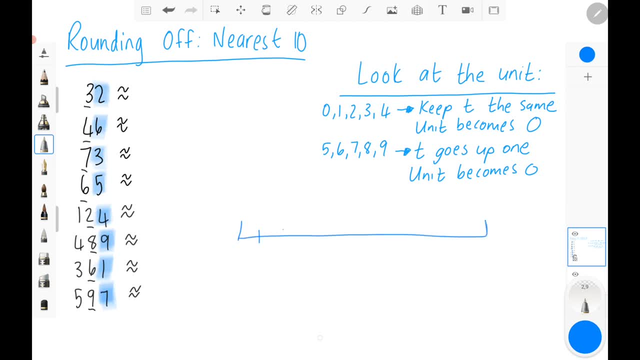 So here's a number line and I've got the numbers 1,, 2,, 3,, 4,, 5,, 6,, 7,, 8,, 9,, 10, okay, I know they're not really well spaced out. 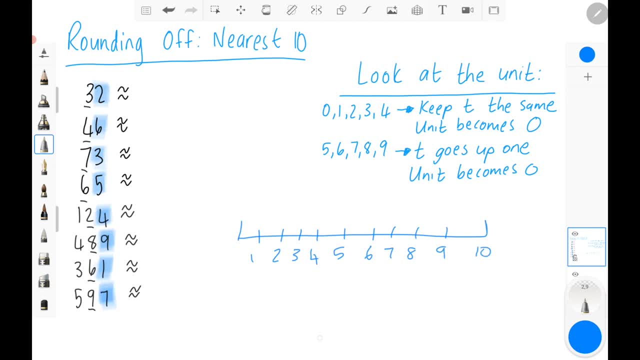 But the whole purpose of this rounding off to the nearest 10, is when you're given a number, you've got to say which 10 it's closest to. Okay, let's say we got the number 7,. okay, And if you had to look, where is the 7th closest to? 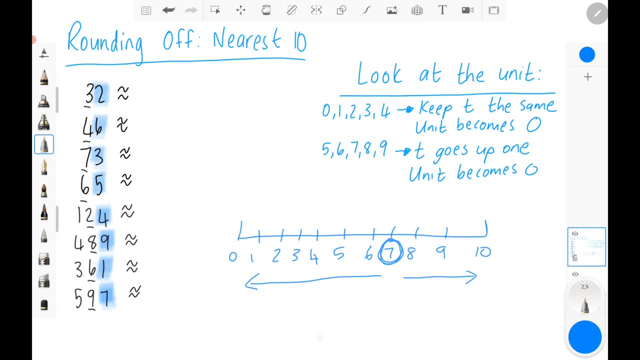 Is it closest to the 0, or is it closest to the 10?? Well, obviously, 7 is closer to 10 than it is to 0. So 7 would round off to the nearest 10,. okay, Well, let's say this wasn't 10.. 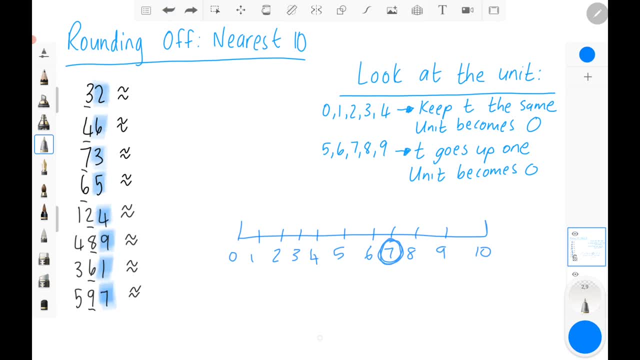 Let's say this was actually something else. Let's say, this was 50. And that was 51,, 52,, 53,, 54,, 55,, 56,, 57,, 58,, 59, and 60.. 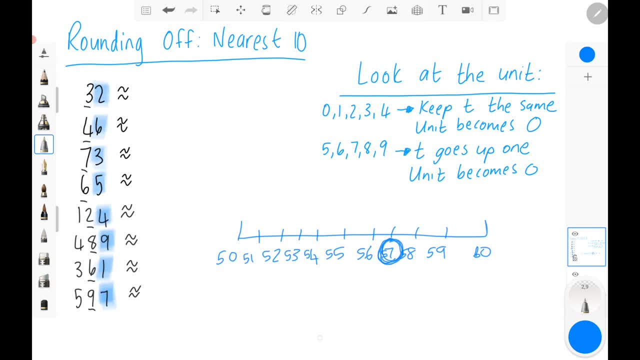 And we were looking at the number 57, and we wanted to know the nearest 10 there. Well, the two 10s that it's in between is 60 and 50. Because if we're counting in 10s and we go, 10,, 20,, 30,, 40,, 50 would be here, 60 would be there. 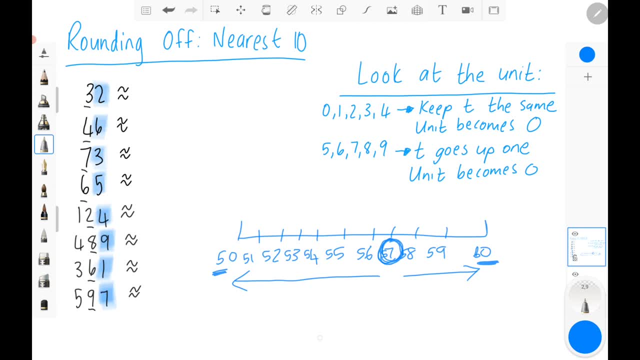 And if we're counting in 10s, which 10 would 57 be closest to? Well, it would be closest to 60. So the point of rounding off is to see which 10 a number is closest to And instead of drawing number lines out like that all the time. 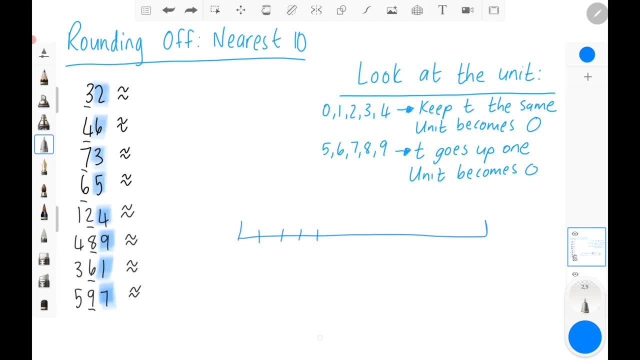 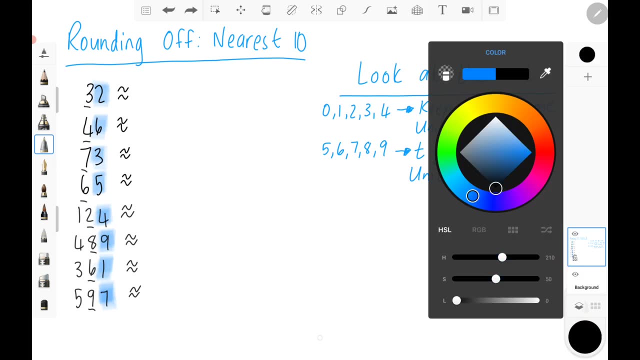 it's going to be much easier for us if we just sort of follow the rules in understanding how to round off. And these rules are what I've written on the right-hand side here. So let's give it a go. You know, once you understand the rules and once you remember the rules by heart. 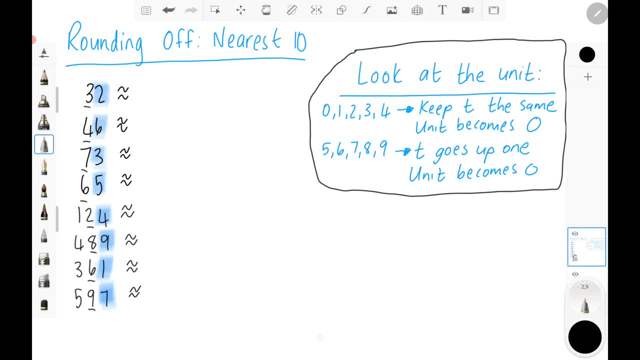 this is going to be a lot easier for you. But if you don't know rounding off by heart, this is going to be a lot easier for you. But if you don't know rounding off yet without looking at the rules, you're going to need to use it when you're figuring things out. 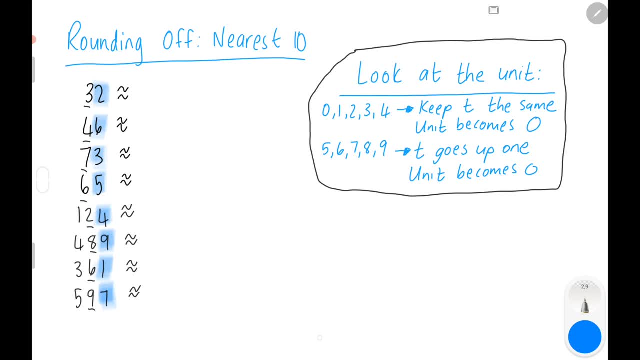 Okay, Now let's look at the first, number 32.. The 2 is highlighted and the rule says: look at the unit. Now where's the 2 fitting? Is it in the 0,, 1,, 2,, 3, 4 side, or is it in the 5,, 6,, 7,, 8, 9 side? 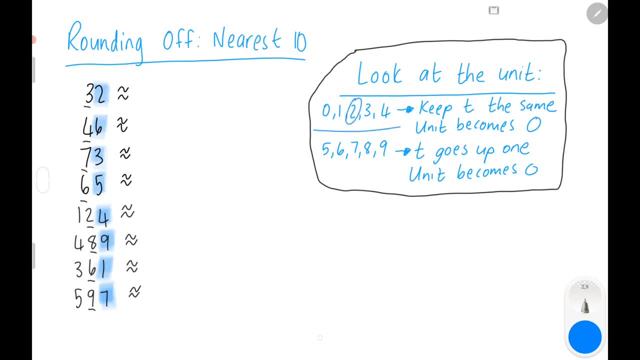 Well, obviously it's fitting here, because that's where 2 is. And if the unit is 2,, what does it say? Keep the 10 the same. My 10 is 30, so I'm going to keep the 30 the same. 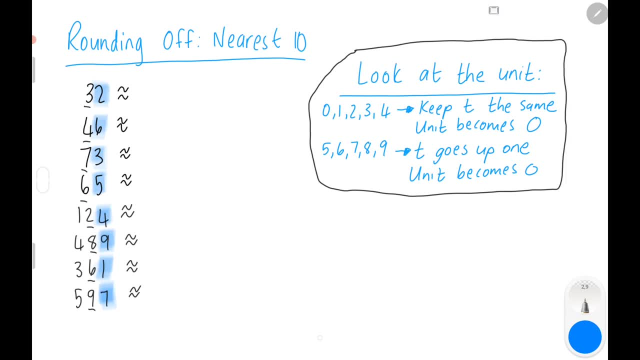 And the unit becomes 0. So let's do that. I'm going to keep my 30 the same. My unit becomes a 0. And what do I get? I get the number 30.. So 32 rounded off to the nearest 10 is 30. 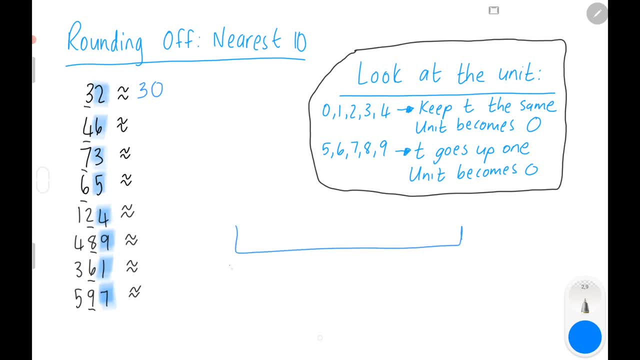 Now that means if I had to put a number line, and here was 30 and there was 40, the number 32 would be much clearer, Closer to 30 than it would be to 40. And this is the point of this whole rounding off thing. 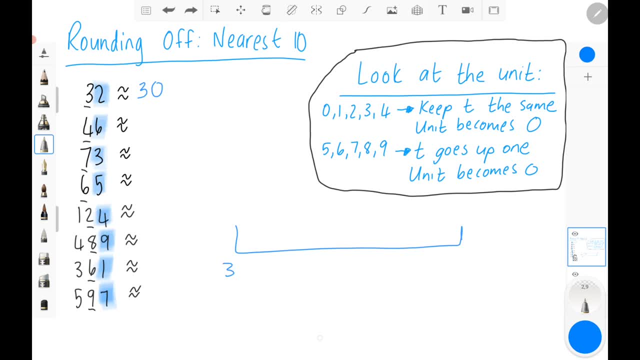 What is it closest to? So let's look at the next one. We have 46.. Where does the 6 fit in in our rule table? Well, it fits in here. And what does it say If it's a 6, the 10 goes up 1, and the unit becomes a 0. 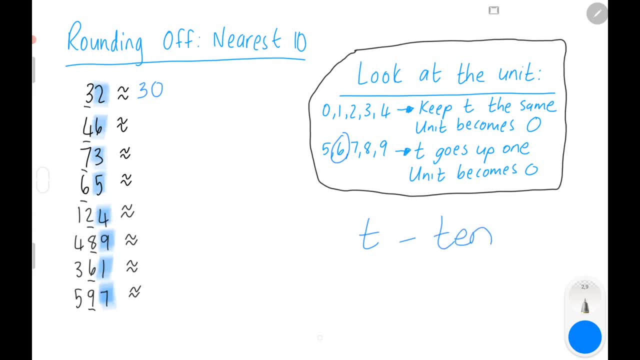 The T, by the way, guys, that stands for 10.. The unit becomes a 0.. Okay, so let's have a look. The 10 goes up 1.. What is my 10 currently? Well, it's 40.. 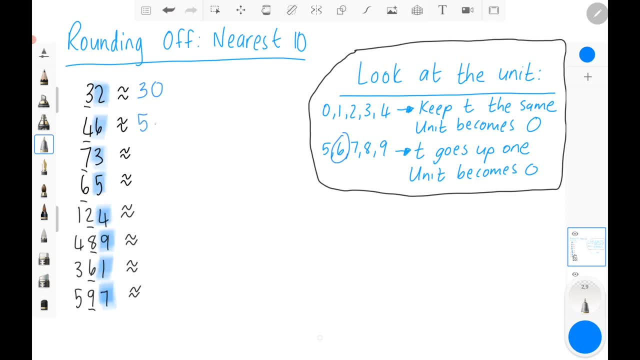 So that 40 is going to go up 1.. The 4 is going to become a 5. And the unit becomes a 0. So 46 rounded off to the nearest 10 is 50.. Good, All right, Let me just take away that 6 that I just highlighted over there. 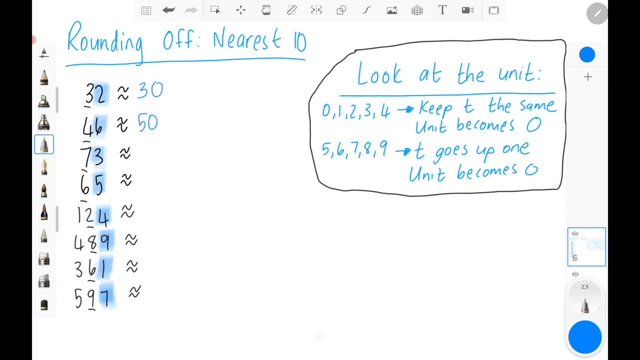 50.. Let's look at the next number: 73.. And where is 3 sitting? 3 is sitting in my top rule, And that is: keep the 10. the same Unit becomes a 0.. My 10, or number in the 10's place, it's a 70 or a 7.. 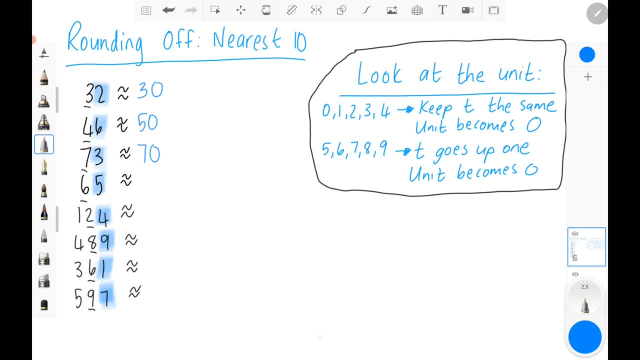 So that stays the same Unit becomes a 0. And it's easy as that: 70., 65,. well, the 5 is sitting in the second rule, And when it's a 5, the 10 goes up 1.. 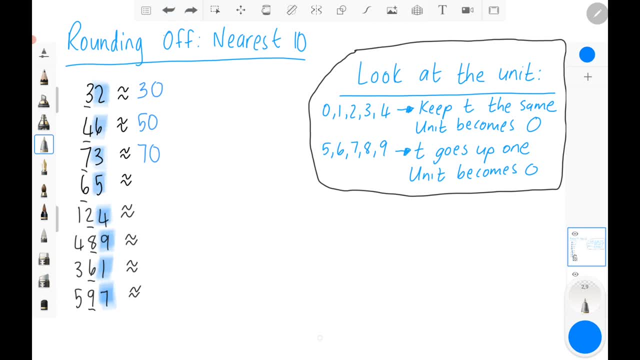 The unit becomes a 0.. What is the 10? currently It's a 6.. So that 6 is going to go up 1 to 7. And my unit becomes a 0. So 65 rounds off to 70.. 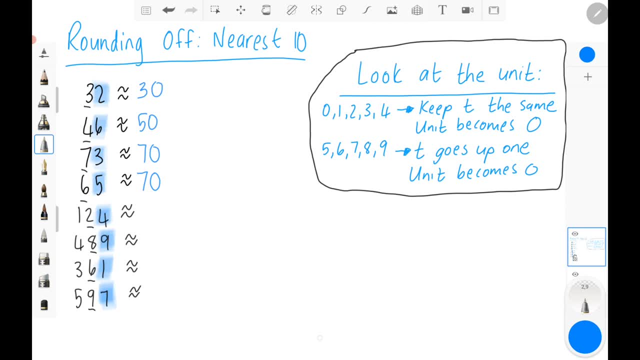 My next number is getting a bit bigger. Now we're moving into three-digit numbers: 124.. Don't let the 100 freak you out, OK, It's just kind of sitting here as part of the number We're doing nearest 10.. 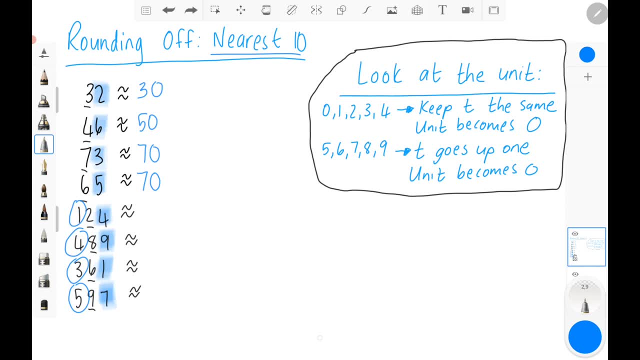 And we're looking at the unit. So the 100 is kind of sleeping. Leave it to sleep, Let it sit there, Let it do its thing. Don't take it away. You've got to still keep it part of your number. 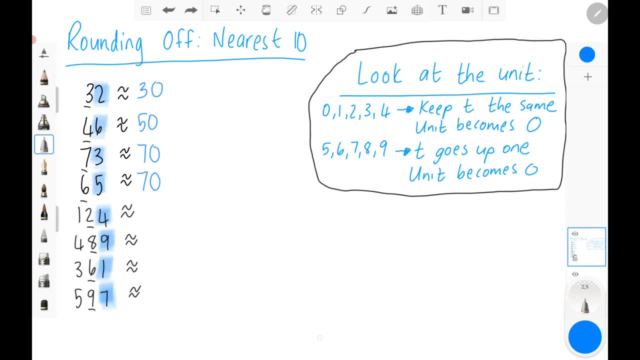 Because the 100 doesn't just disappear into thin air. OK, Let's look at the 4.. Because that's the number we highlighted. That's the unit. We look at the unit. The unit is a 4.. And what is the rule? 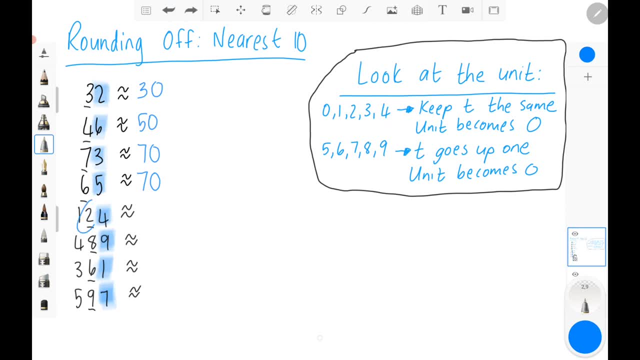 Keep the 10 the same, The unit becomes a 0.. What is my 10?? Well, it's a 2.. So the 2 stays the same, Unit becomes a 0.. And, guys, we bring back the 100.. 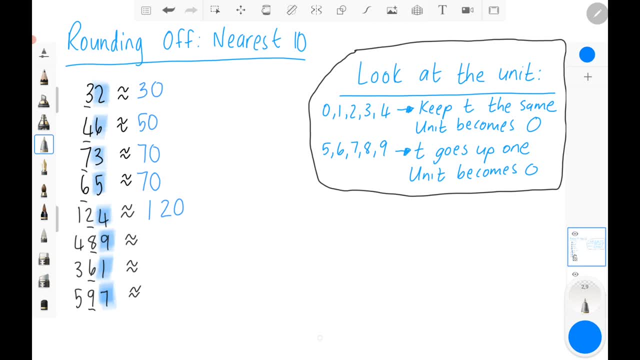 We leave the 100, the same as well. OK, And when you get up to thousands, which I'll show you just now, the thousands also stay. You leave the thousands alone. Let's look at the next one: 489.. What do we do? 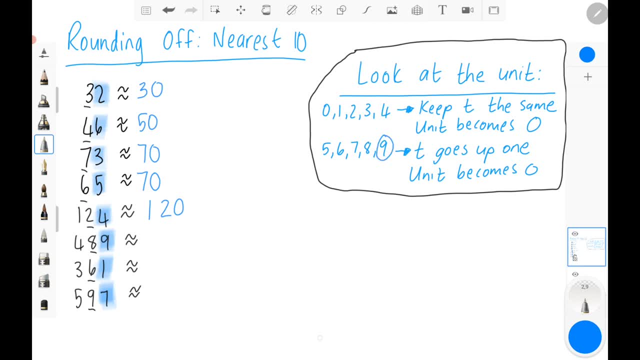 We look at the unit. The unit is a 9.. And what happens? The 10 goes up 1.. The unit becomes a 0.. What is my 10? currently, It's an 8.. So that's going to go up 1.. 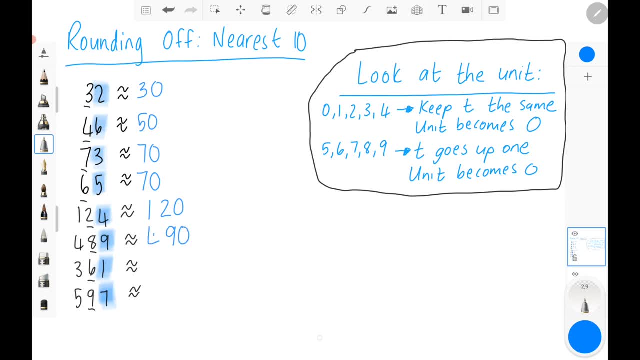 It's going to become a 9.. My unit becomes a 0. And my 400 stays as it is, OK. 361.. The unit is a 1.. And what do I do? Keep the 10. the same Unit becomes a 0.. 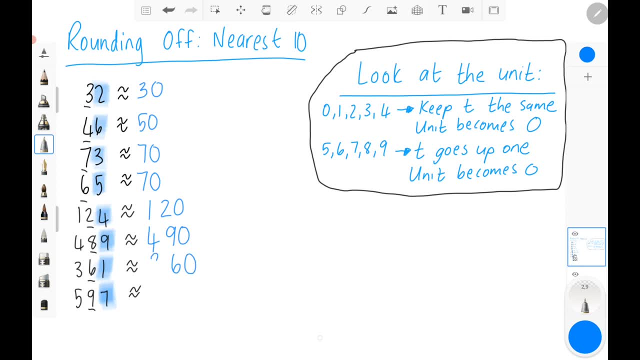 The 10 stays a 6.. Unit becomes a 0.. My 3 stays, as it is, The 300.. The last one, guys. Now, this is a very tricky one, So I'm going to put a star on it. 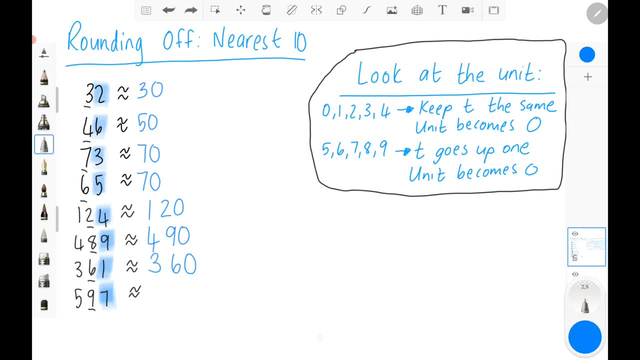 Be careful of things like this, because you'll see what's going to happen now. My unit is a 7.. And when I look at the 7, what does it say? The 10 goes up 1.. The unit becomes a 0.. 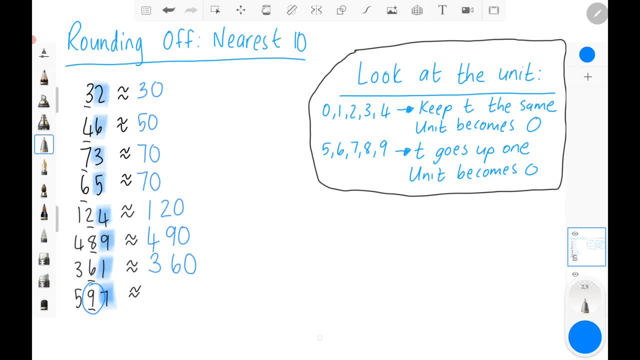 So let's look at what's in my tens column: It's a 9.. And guys, what is above 9?? 10, right, But I can't go writing 10 and then a 5 and then a 0, because what's it going to turn into now? 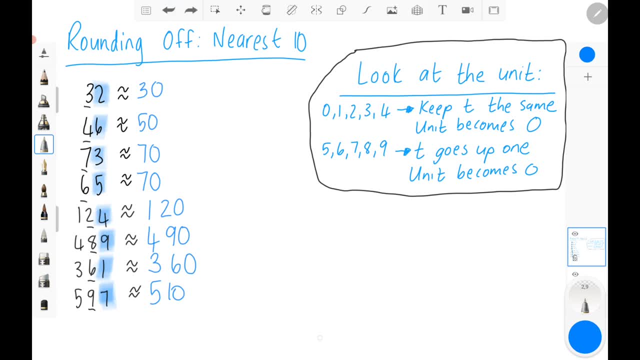 Now it's going to turn into thousands. We know after 90, because, let's face it, what's sitting in the tens column now is a 9.. And when it's a 9 in the tens column it's a 90.. 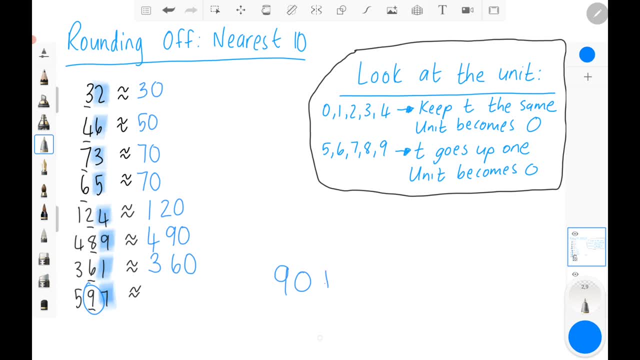 If I add 10 to that, if I go up one 10, what does it become After 90, if I'm counting in tens 60,, 70,, 80,, 90.. After 90, we get 100. 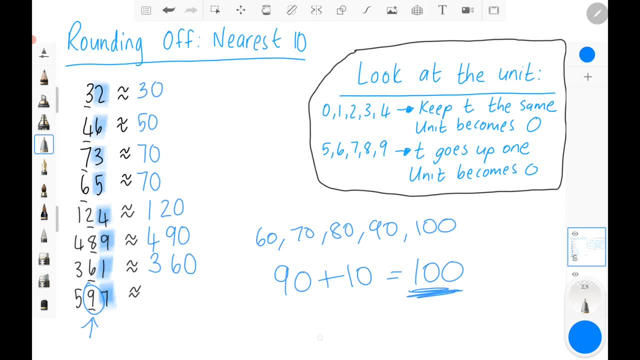 Okay Now, because this 9 can't just go up one on its own. what it's going to do is it's actually going to change the 100 as well. The 100 is going to have to go up one as well, because it's become something into the hundreds column here. 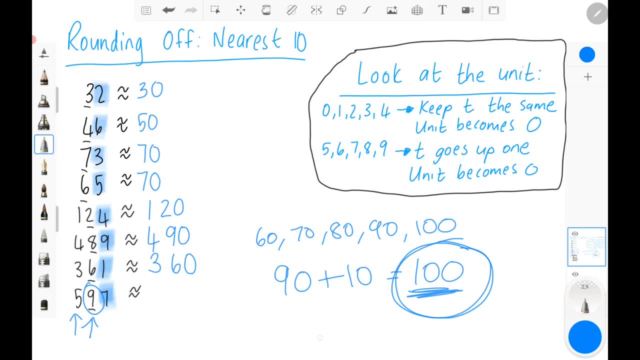 Okay, The next 10 from 90 is 100. Which means, guys, I'm going to have to push that 100 up, And what is sitting in my hundreds column right now It's a 500.. So what I'm going to have to do now is we're going to have to push that 500 up one to a 6.. 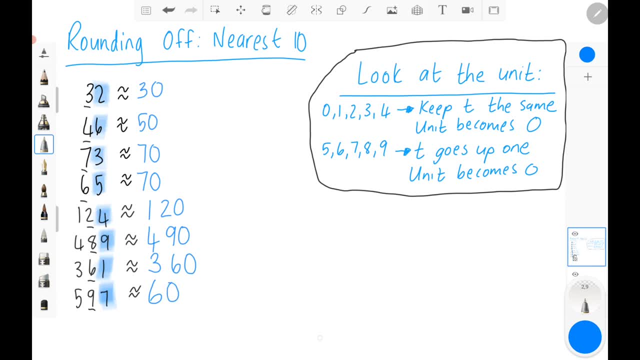 And because 90 went up one into the hundreds, we're going to make that a 0.. And our unit becomes a 0.. Okay, So 597,. the closest 10 to that will be 600.. These are the tricky ones. 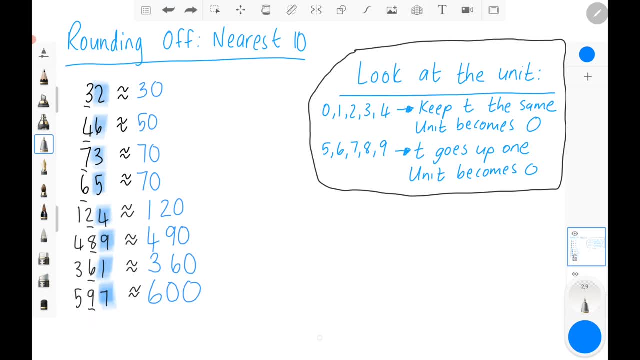 We're going to move the next one up one. Okay, Guys, if you are sitting now at term 3, you will have been doing thousands, And I just want to show you what thousands are about. If you're not in term 3, don't come and have a look at this video. 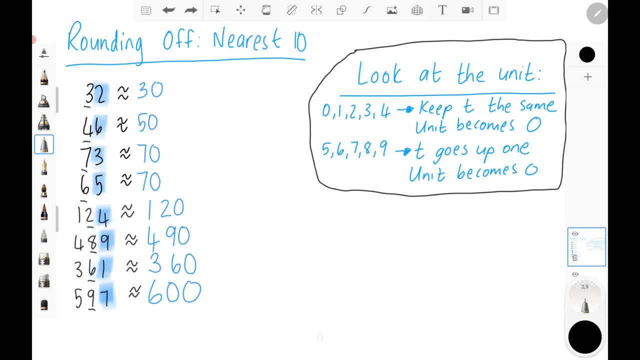 But if you are in term 1 and you want to know about thousands, then stick around And you can learn a bit about thousands. So I'm going to give you four examples of what would happen if we start introducing things in the thousands place. 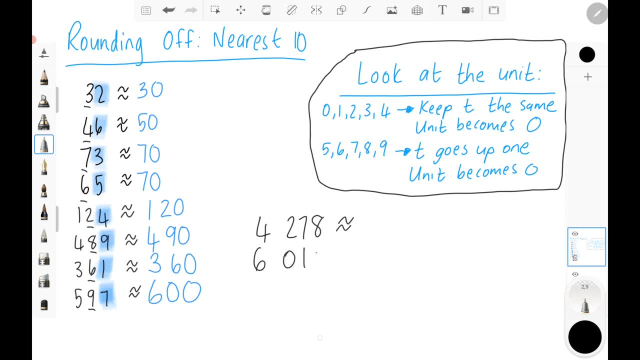 And what would happen if you've got thousands? And what would happen if you've got things in the thousands? Okay, So let's do that, And I'm going to do one more on the side here, All right, So what's the first thing we need to do? 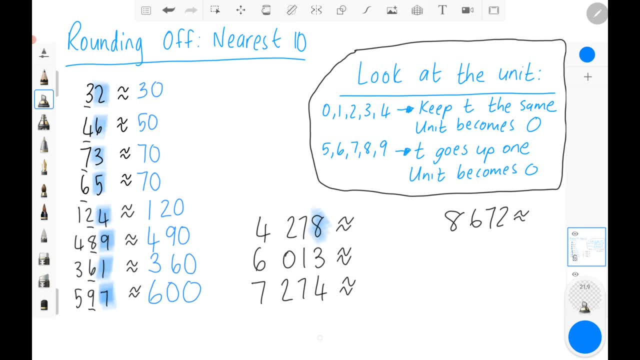 Look at your unit. So immediately I'm going to highlight my unit And what is the thing that needs to change? It's nearest 10.. So we're going to underline our 10s and say, okay, that's the thing I need to change. 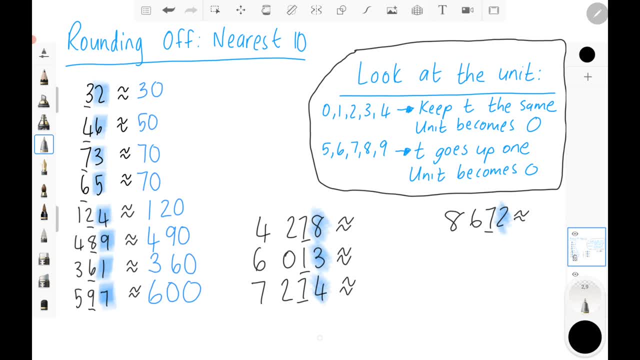 Now we look at the rule. Look at your unit. The first one over here is an 8.. Let me just get my blue pen. What happens when we have an 8?? The 10 goes up 1.. The unit becomes 0..